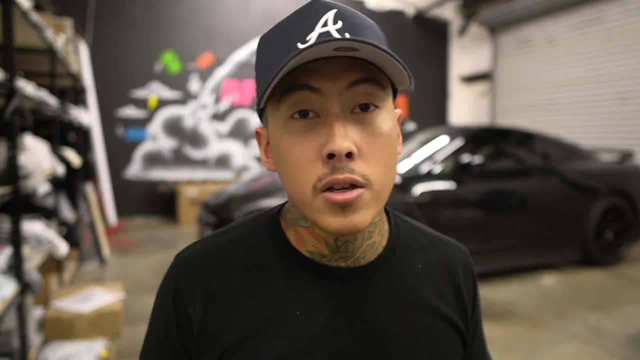 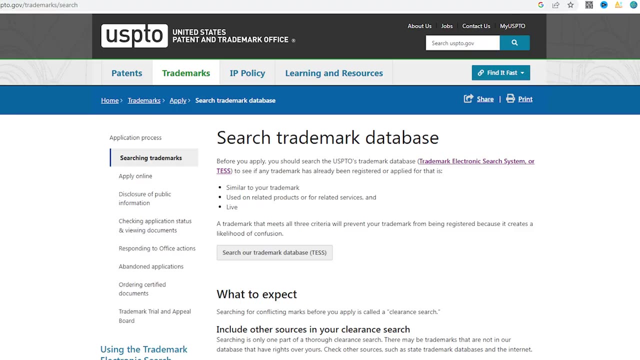 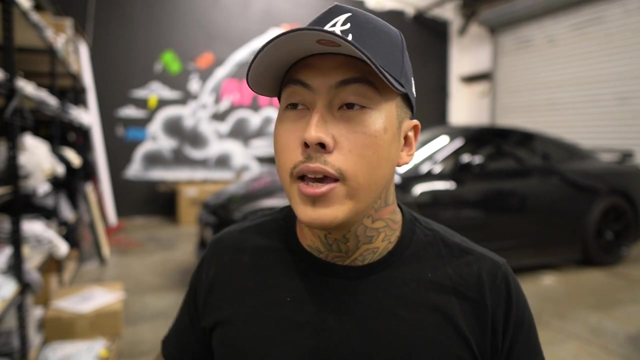 experience. the only thing I've ever done is trademark things. You can always go to usptogov- That's the trademark office- And you can also go on here to search, to even see if your trademark has been used, And most of the time for us we have to see if it's been used in the clothing. category. So in about 2015,, 2016,, I attempted to trademark something myself on the trademark website And I went directly on the website and I attempted to trademark something myself And I signed up and I paid. I can't remember exactly, but I think it was like $100, $150 to. 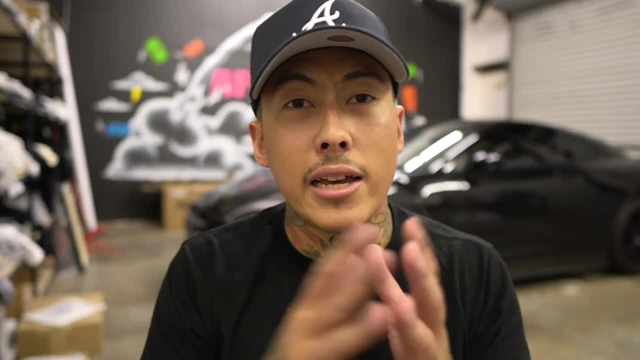 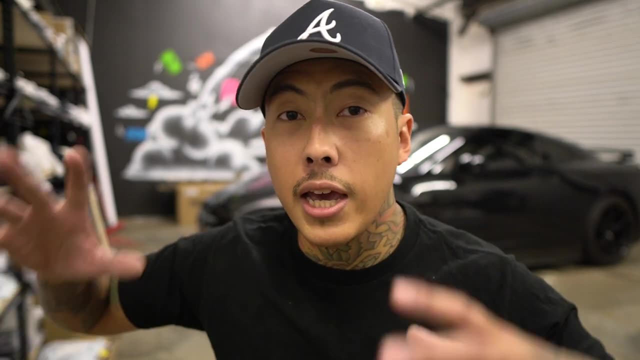 file it And you have to gather your specimens, anything and everything that's related to your brand, and upload that as well. And whenever you trademark it, it goes towards the office, right, And the office can reject it because it can be confused with other brands. that's not even. 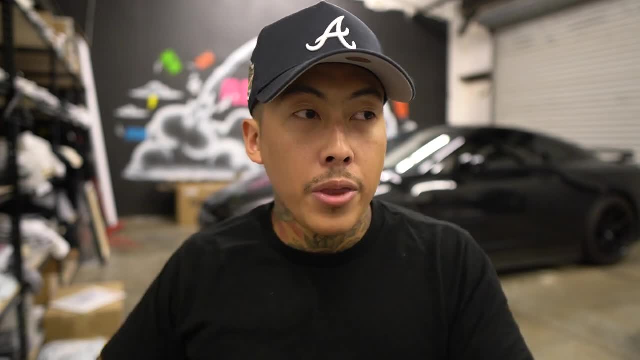 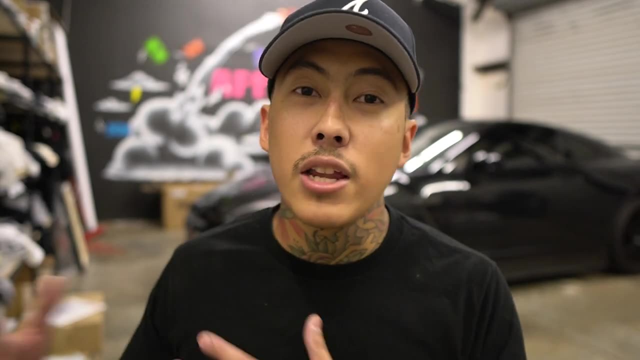 necessarily in your category of trademarks. So at that point in time, it was either I could abandon it or I couldn't do it, And so I signed up and I paid. I can't remember exactly, but I had to respond in a proper fashion, which I really didn't know how to do so. So that was my first. 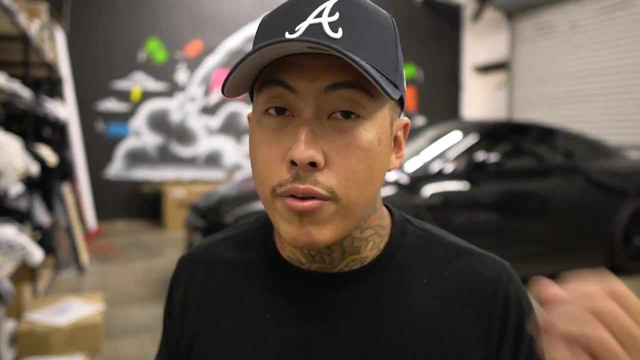 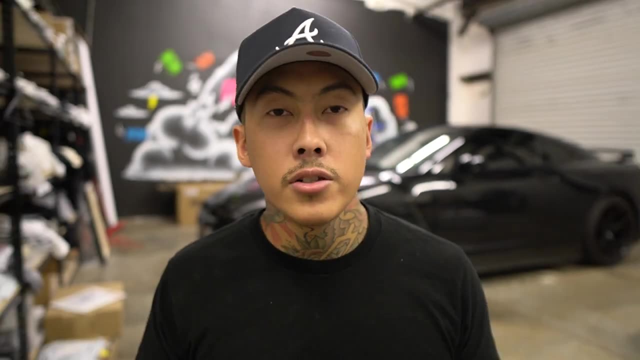 experience. I just left it abandoned because the information that they provided back was really confusing with the brand that I had with other brands that was also out. So the second, third and fourth time around I pretty much just used LegalZoom. You could go directly to a trademark. 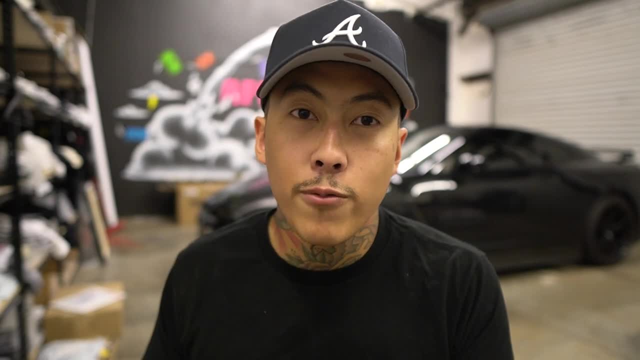 attorney as well, but LegalZoom was just an easier way for me to do this. This video is not paid by LegalZoom. It's not paid by LegalZoom. It's not paid by LegalZoom. It's not paid by LegalZoom. It was easier for me to do this. I just went on their website. It was like 600 bucks And that's just to be able to use their attorney- And you type in the information that you want. still, go to usptogov and use their search system to make sure that it's something that you can trademark. 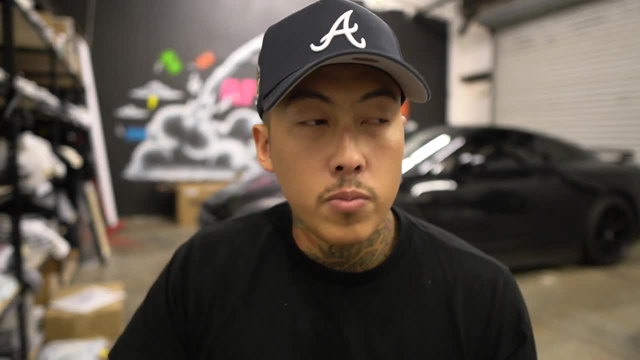 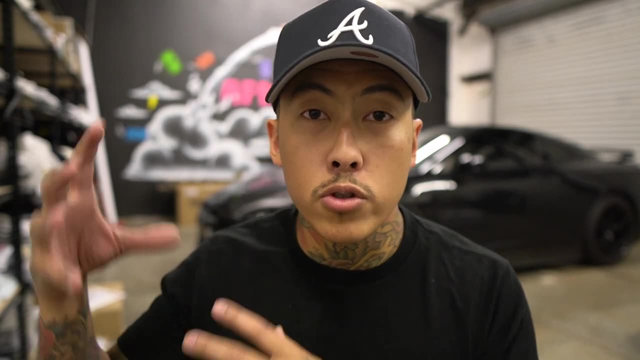 first of all- and it's not taken, But I went to LegalZoom and once you pay that $600, you'll go through a intake call and you'll talk to someone from LegalZoom then and they will explain to you what you need. 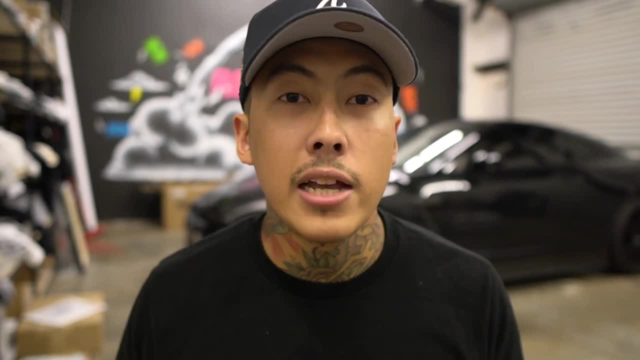 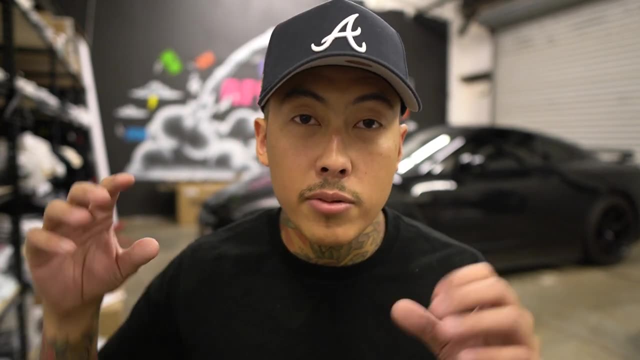 Before you talk to the attorney. then you get to talk to the attorney and you let them know what your brand is and then they will file the trademark for you. So if usptogov, the trademark office, comes back and say something about the brand, they're able to respond to it properly. 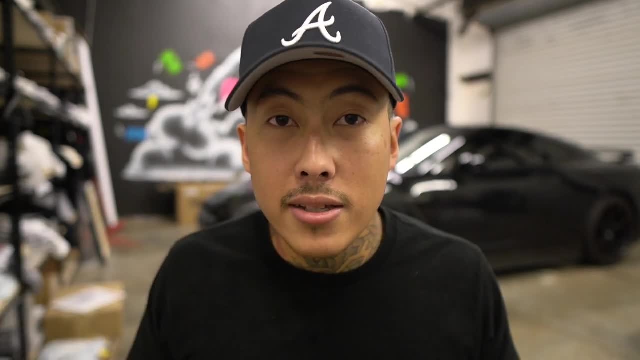 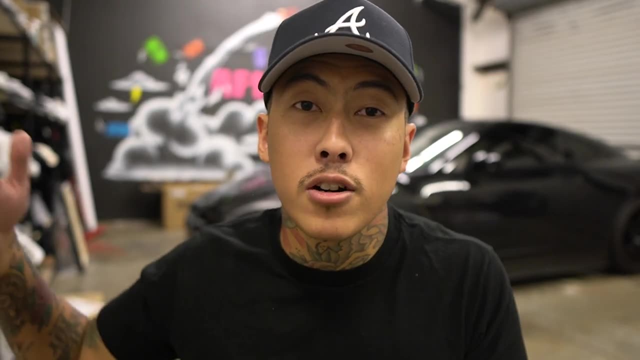 more knowledge that I have. So this made it more easy for me. but you have to pay that $600 on top of still that filing fee, which is like 150 bucks or so. So for me that $600 was more worth it.